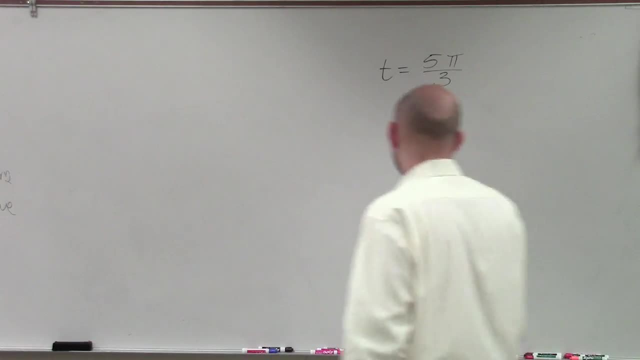 So in playlist one, two and three, I describe how to first start writing an angle. So the first thing we need to do, ladies and gentlemen- actually there's three things we're going to do- First thing we need to know is again: 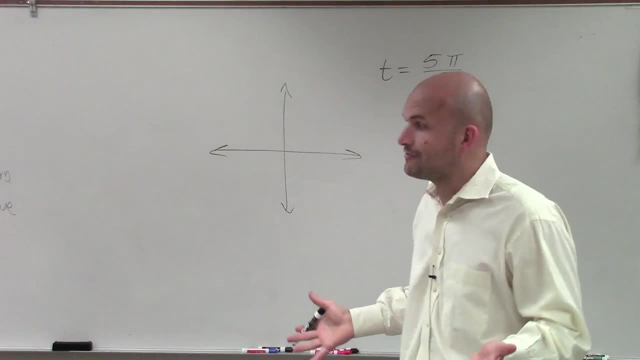 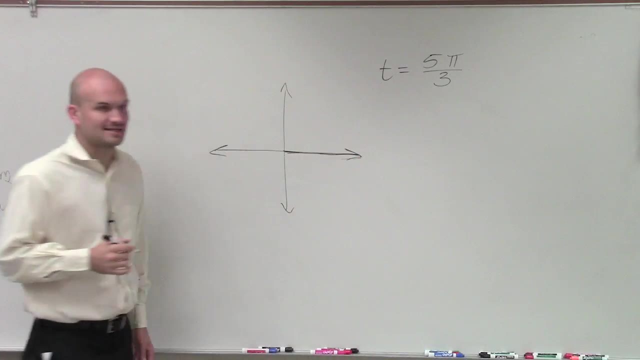 what exactly is an angle right? What is this? t equals 5 pi over 3?. Well, remember, when we're doing an angle, an angle has two sides. We have our initial side, which is going to be on the x-axis. 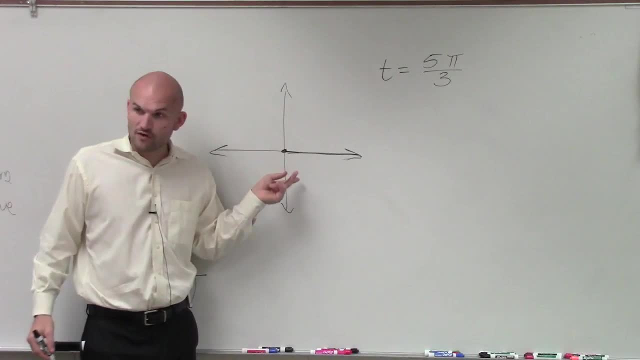 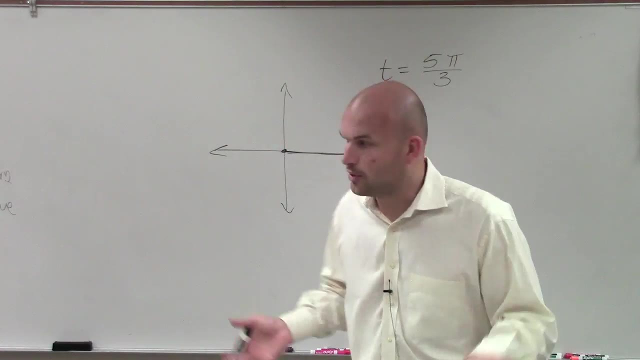 Then we're going to rotate a secondary ray off of our vertex from there and that's going to be called our terminal side. But we need to be able to determine what is then. where is this point or where is this 5 pi over 3?? 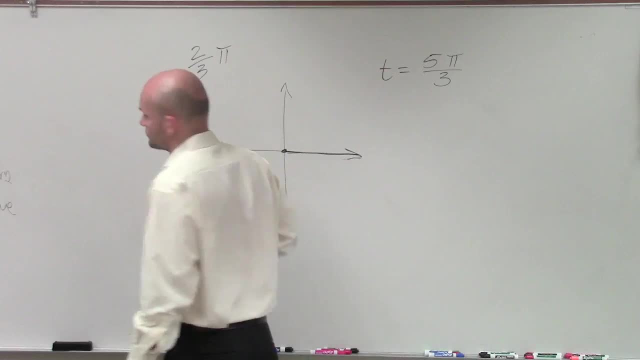 So let's go and look at 2 thirds, 2 thirds pi, All right, And let's forget. let's talk about pi. Let's talk about a dollar bill, right, If I say I have 2 thirds of a dollar. 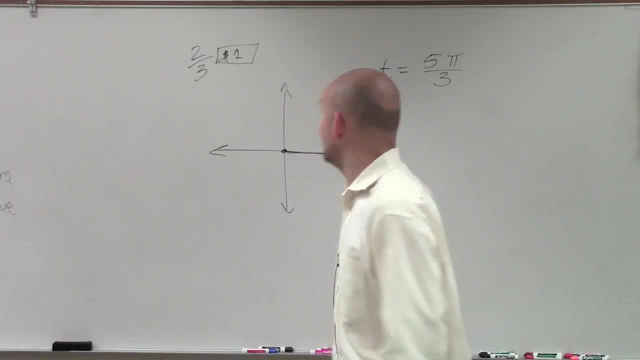 do I have more or less than a dollar Less If I say I have 5 thirds of a dollar, do I have more than a dollar or less than a dollar? More right, Good, So now let's go back to pi. 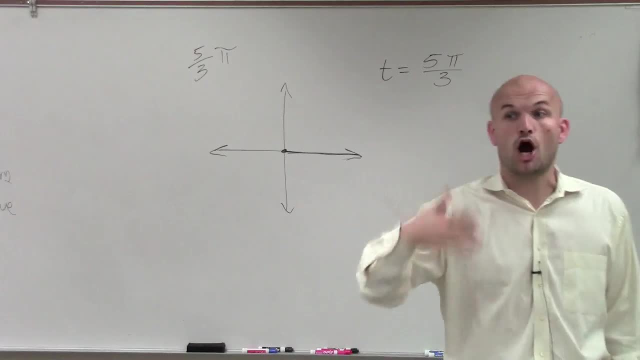 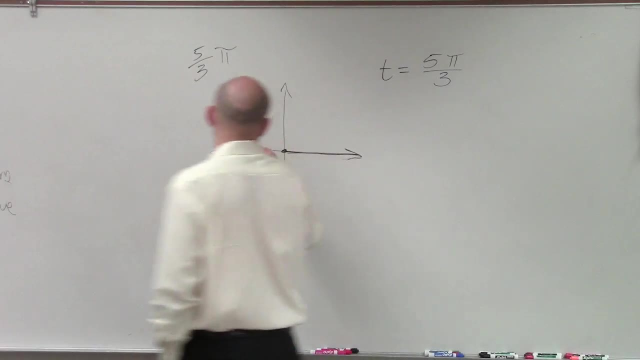 So if I have 5 thirds of pi, that means I have an angle that's larger than pi, correct? All right, so now we need to go back and remember well, where does pi exactly come from. So we go to our point of pi. 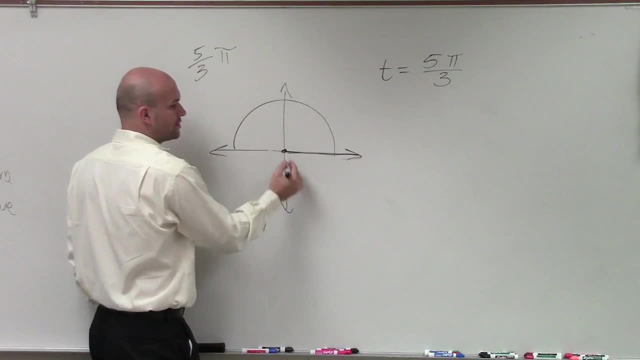 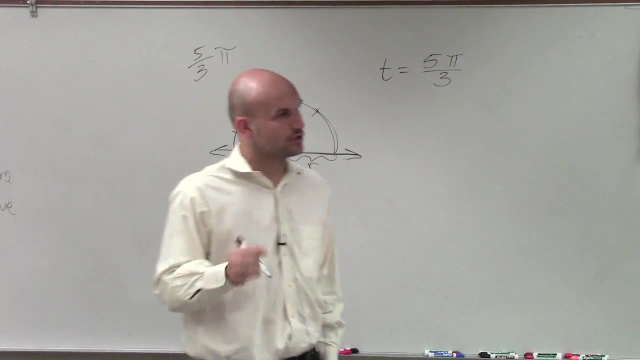 Remember what it took from our unit circle. When we have a circle we have a distance which we call the radius, And if we wrap that radius around a circle, we can wrap the radius around the circle three times, but we don't get it all the way. 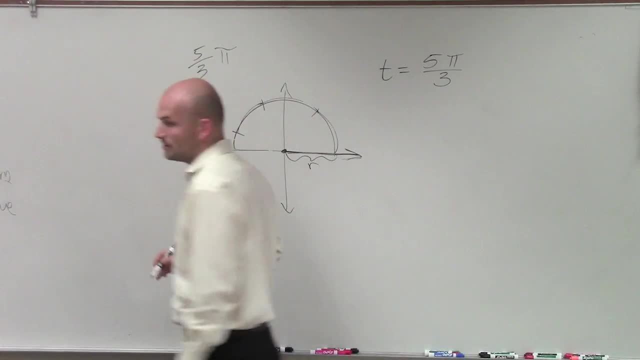 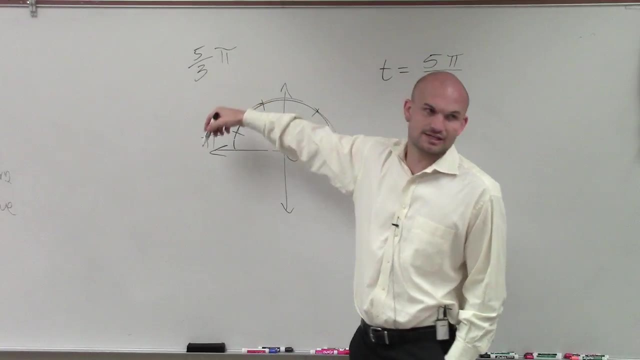 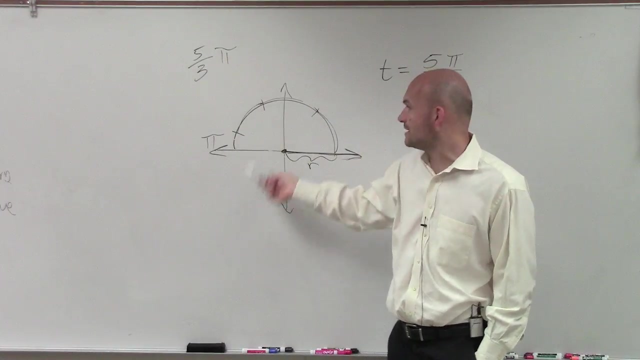 There's that little chunk that's extra, which is a decimal, irrational decimal, going on and on and on, Which is 3.14159, so it's pi. So we know this distance in degrees is 180 degrees, But in radians, in terms of the radiuses wrapped around it. 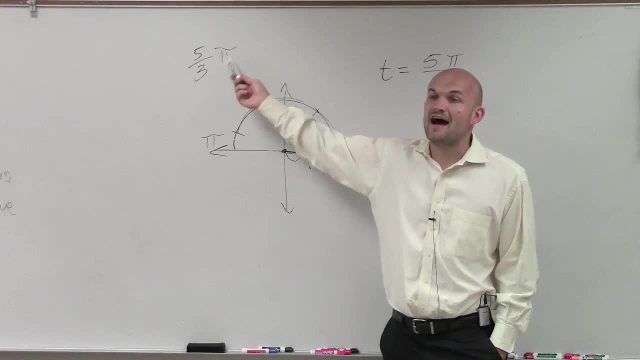 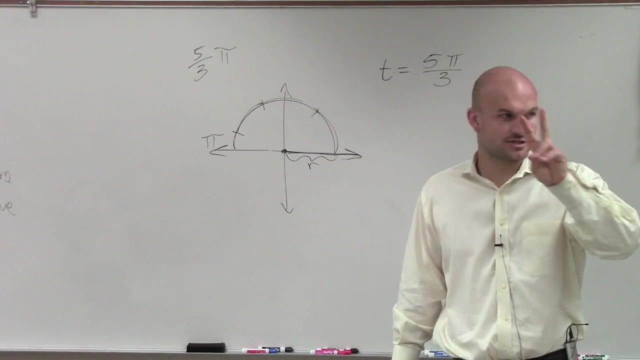 it's pi radians. So I have 5 pi over 3,. right, I have an angle that's larger than pi, But how much larger. It's 2 thirds larger. right, I have two extra parts. So what I like to do when I'm trying to describe 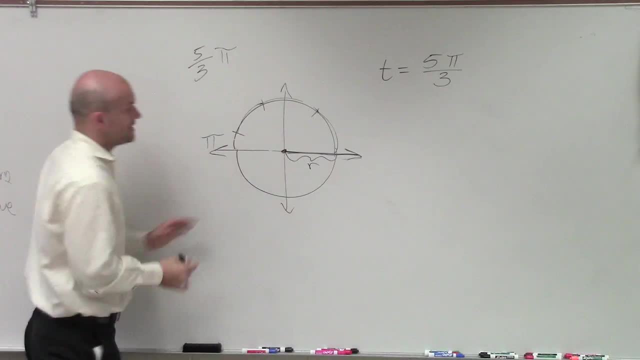 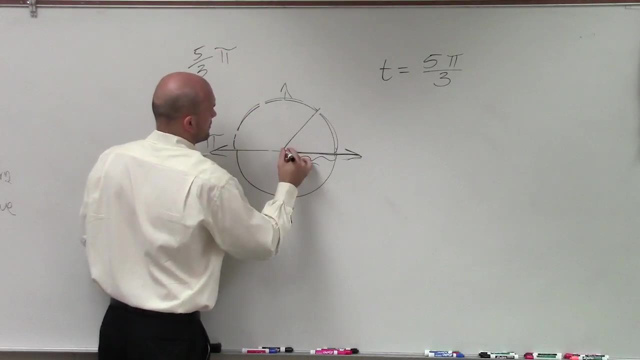 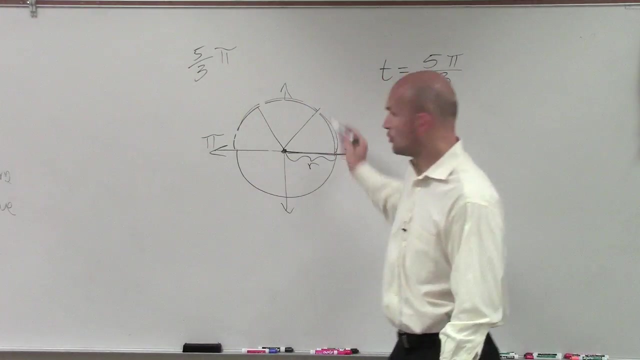 where this angle is. what I like to do is I like to take a look at my denominator and break up my pi into that denominator. Does everybody see how I now broke up pi? the distance from here to here? I broke it up into thirds. 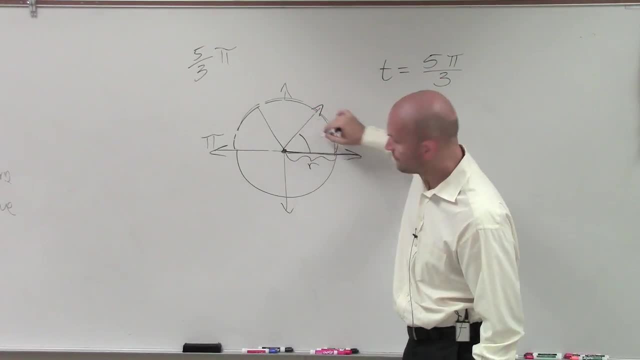 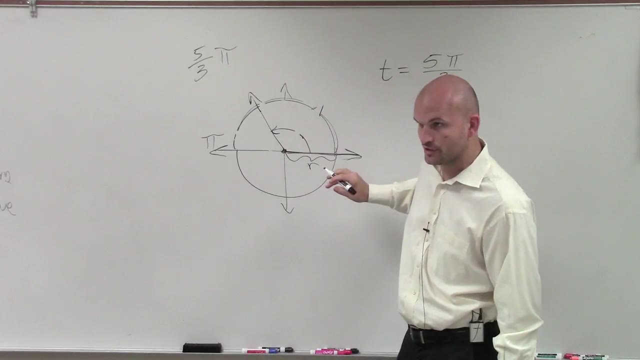 So you could say: well, if I had two angles from here to here, that would be 1 third right. If I did my angles here, if I did from here to here, that would be 2 thirds right, And all the way around would be here. 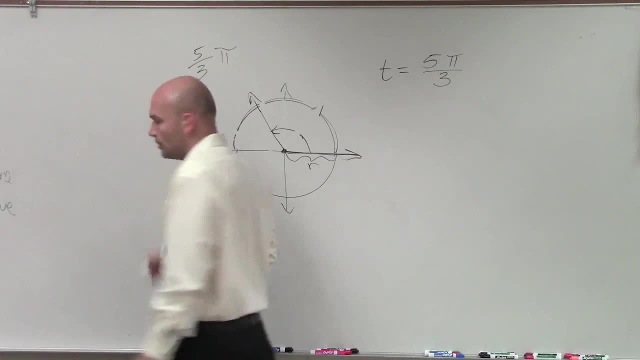 That would be 3 thirds, So this is the same thing as 3 pi over 3.. Does that make a little sense? Israel, you got it Good. So the question, though, is actually: we can do this again on the bottom? 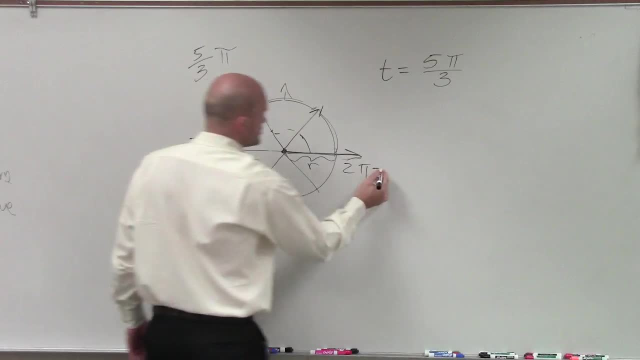 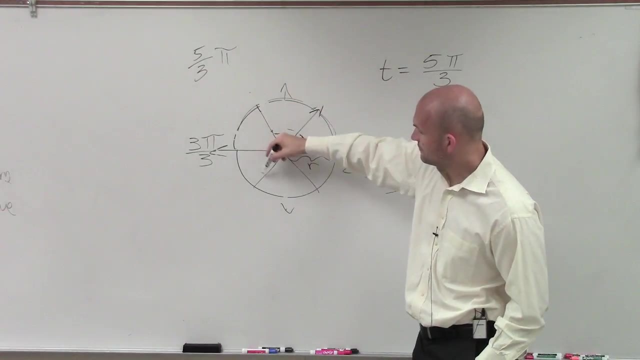 Because, remember, wrapped around all the way around a circle, is 2 pi, which in this case would be 6 pi over 3, right, Because 6 divided by 3 is 2.. So 1 pi, 2 pi, 3 pi, 4 pi, 5 pi. 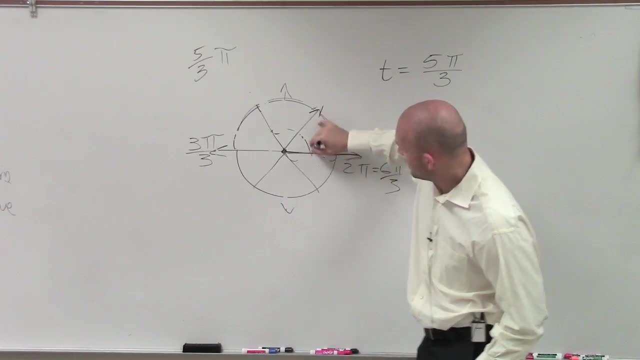 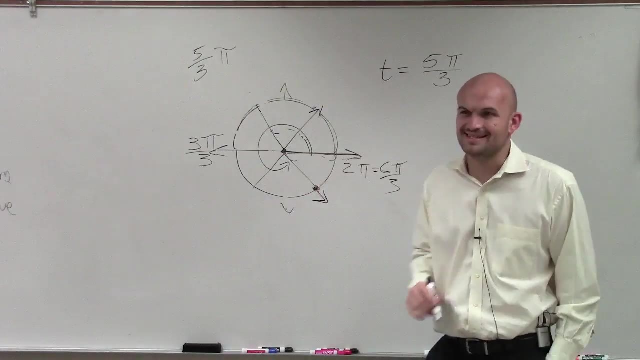 So here's my initial side, And I wrap all the way around to here. So there's my angle. Now what I need to do is determine: where is this point? What is that point on the unit circle If I have an angle at 5 pi over 3,? 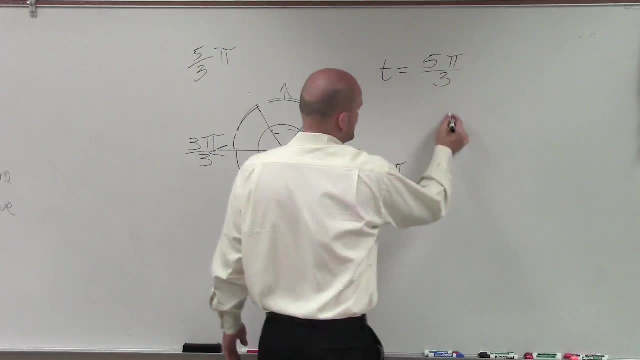 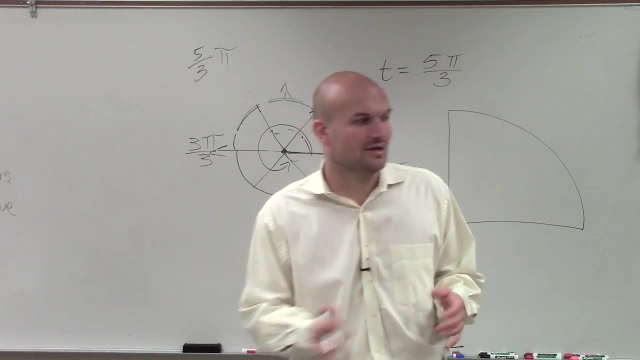 what point is that? on the unit circle. So then I go back to the playlist on what is the unit circle. And when I talked about memorizing the unit circle, I don't care about you guys knowing the whole unit circle. I care about you knowing what the first quadrant is. 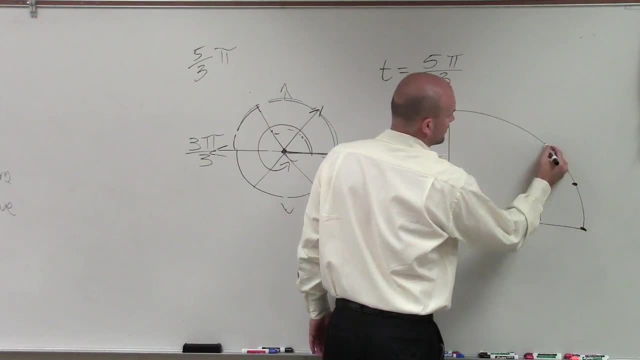 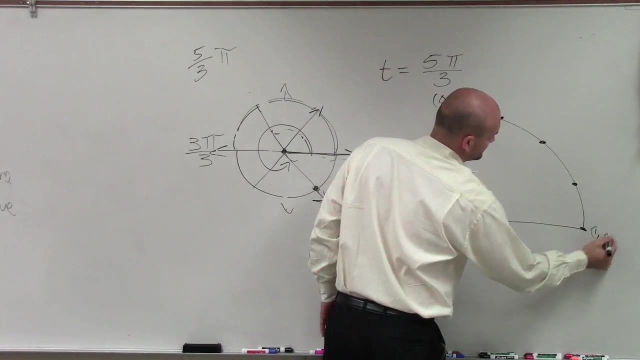 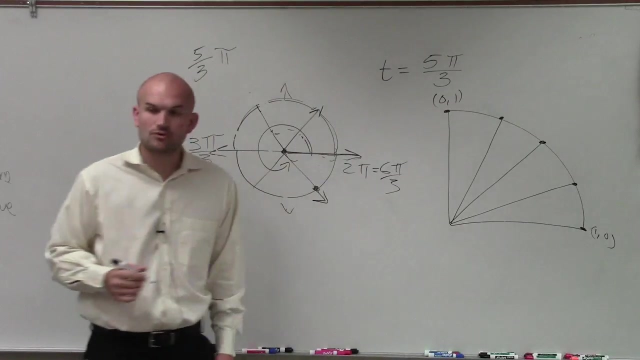 In the first quadrant there was five points that I deemed were the most important: 0 comma 1, 1 comma 0, all right, And then these other points were off of angles that we found from special right triangles. The first angle, which was 30 degrees, 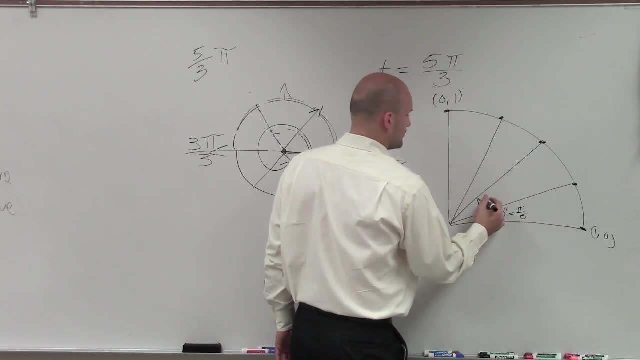 which is equal to pi over 6.. The second angle, which is 45 degrees, which is the same thing as pi over 4. And the third angle, which is 60 degrees, came from pi over 3.. All right,